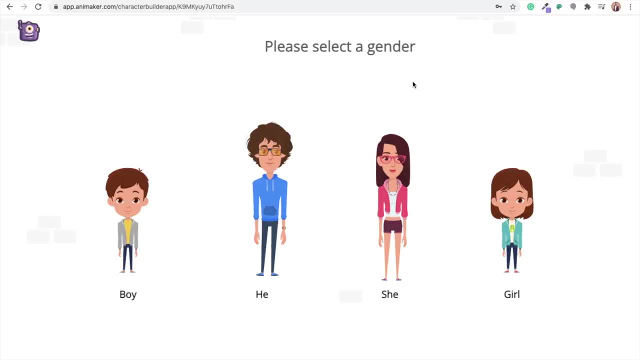 option. It will open the character builder of the animaker. Before starting to create the character, keep a picture as a reference. I am going to use this girl's picture as a reference and recreate it. You can use any of your own images. Choose the character's. 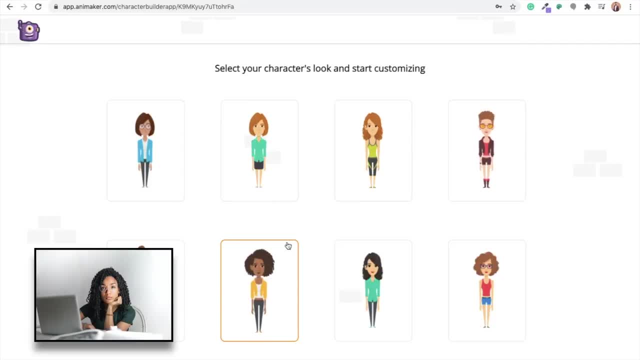 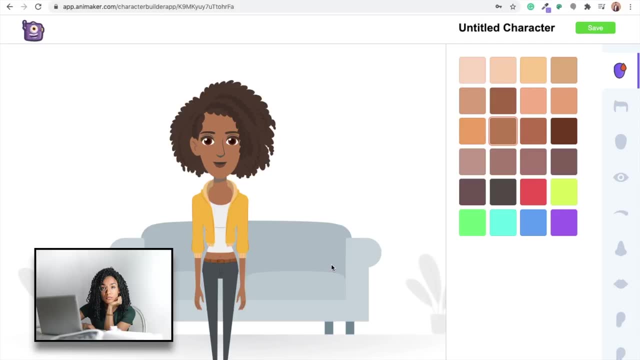 gender. Choose a basic template that resembles your picture. I think this character over here looks the most similar to the image we have, So I am selecting this one. You can change the color of the skin. Then we have options to change the different facial features. 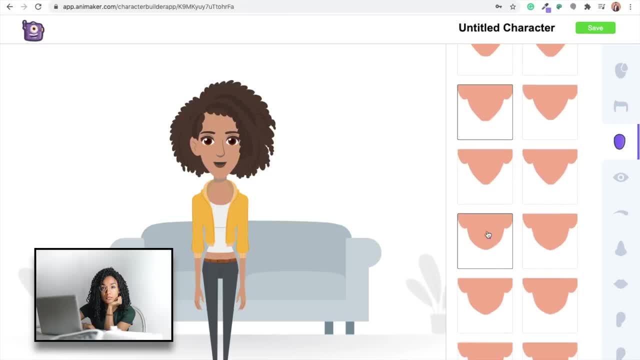 like shape of the face: eyes, eyebrows, ears and so on. Change each of these features to match the picture. Using all these options, you can literally create billions of unique characters. Now let's move to the attire. The color of the dress in the picture is green, So let's. 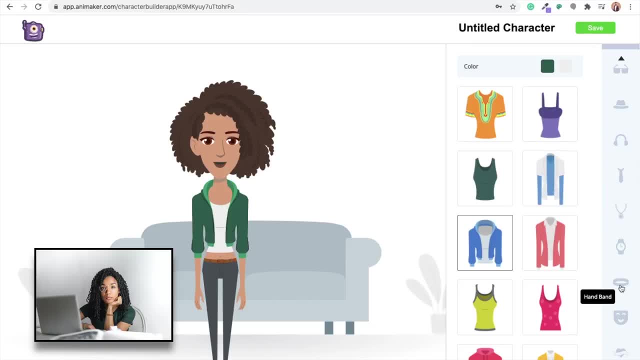 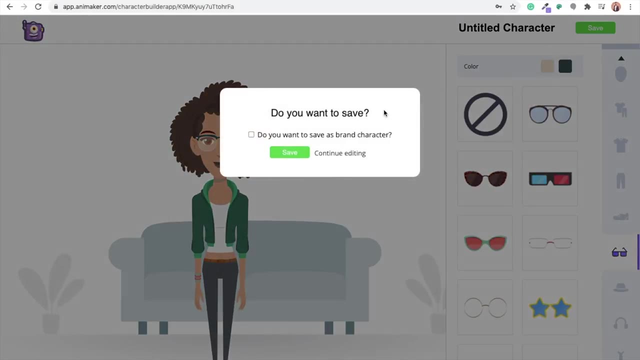 change it. Let's swap on the wearables. This character is wearing a hand band, So let's add it. Let's not forget to add the glasses. Once you have completed creating your character, select the save option at the top to save the character. Now let's see how to use this. 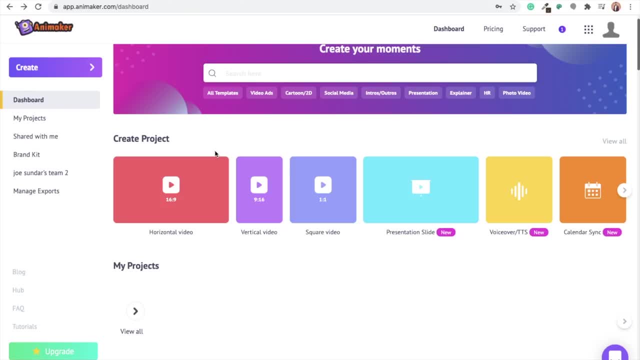 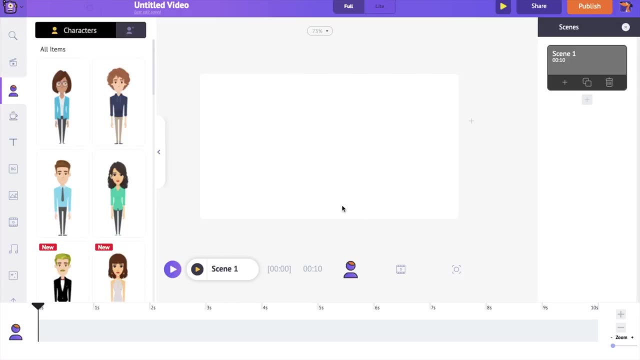 character to create amazing animated videos. Now get back to the dashboard. Select the create option on the left, followed by selecting create a video and blank page, A new project will be created. This is how the interface of the animaker application looks like. At the center, we have the workspace, the place where you will be creating your videos. 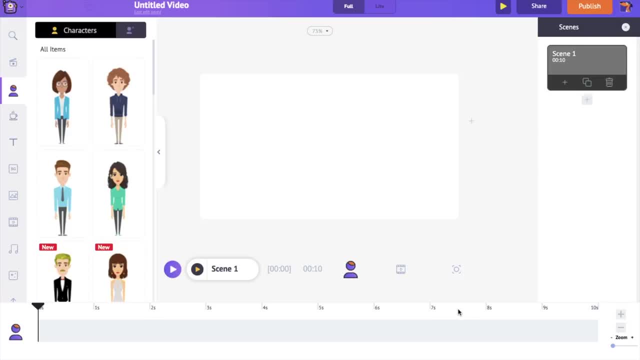 On the right hand side is the scene section. On the bottom is the timeline. Within the timeline you have three different timelines: First is the animation timeline, The second is the video timeline And finally we have the camera timeline On the left hand side. 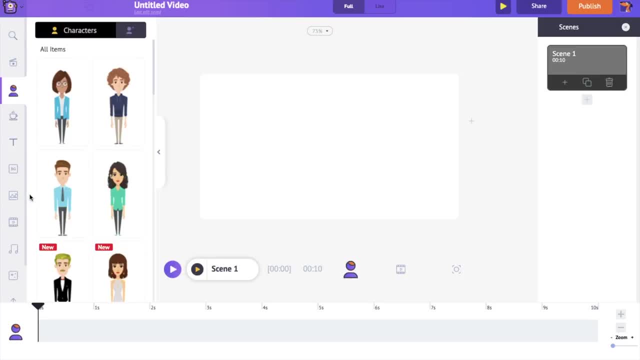 you can see the library, which consists of different elements that you will need to create the video. You can see the character section of the library is open by default And it has a variety of characters, starting from male and female characters. Then we have kids characters. 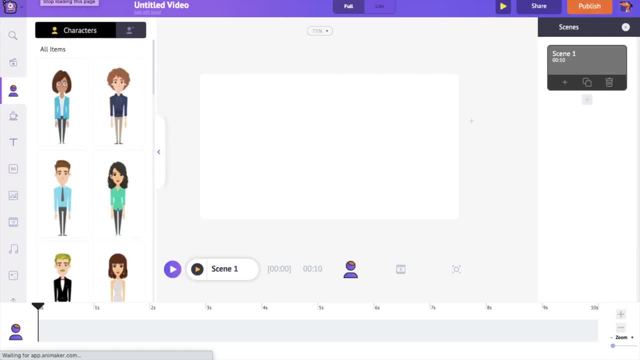 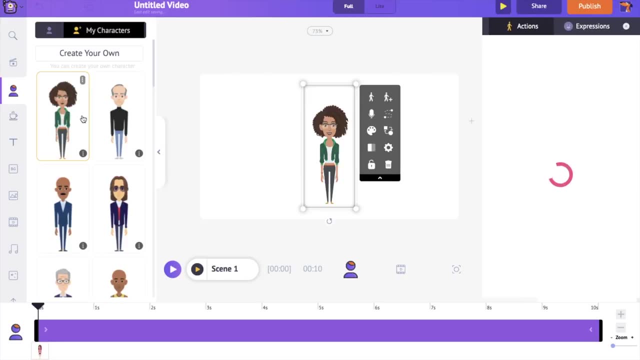 And finally, we have animal characters. You can find the newly created character in the my character section of the library. Click on it. It will appear in the center of the workspace On the right hand side. you can notice the actions tab in open. From here you can apply the actions to the character. Use the search. 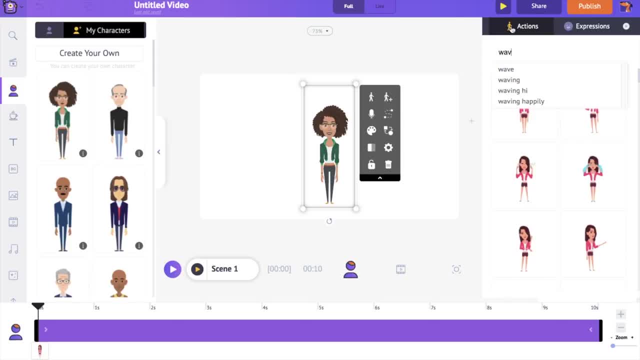 option at the top to find an action. I am going to search for the word waving. Select the action. On the timeline you can notice a purple colored bar. It represents the duration for which this character is going to be visible. If I want the character to appear a little, 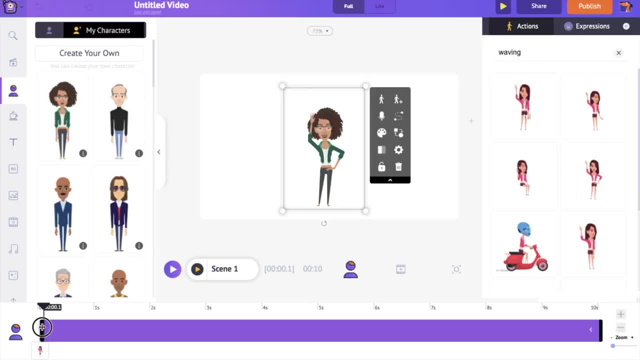 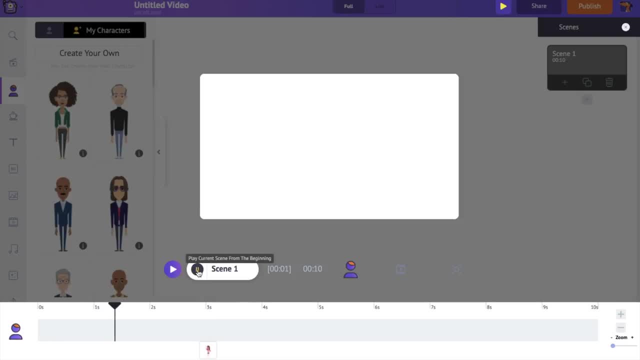 later I have to select the left edge of this bar and move towards the right. If I hit the scene preview option, you can understand how this works. you can also add multiple actions to the same character and create a full-fledged animation video. we have 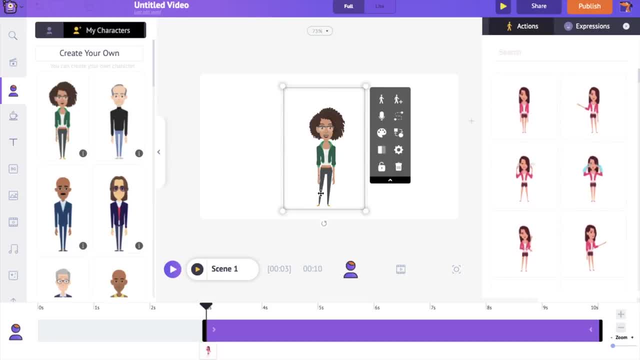 already made a detailed video on how to animate the characters. I am adding link to that video in the description. you can check it out later. right now the background is white in color, but you can add colors to the background. click anywhere on the workspace and now you can see a new option appearing on the 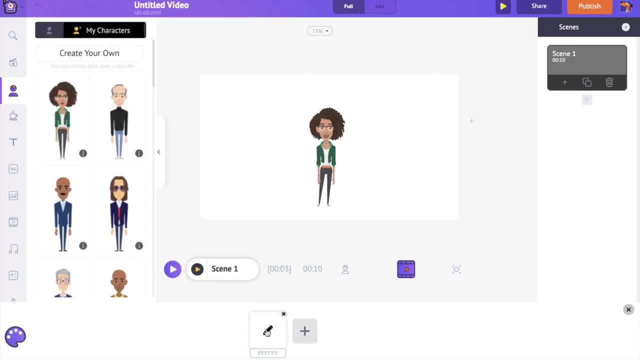 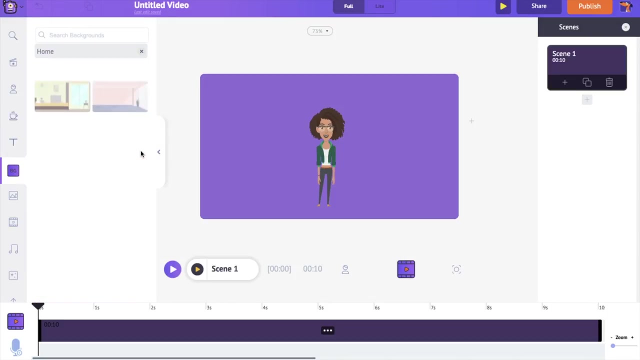 bottom. use the Edit option to change the color. you can also add multiple colors to the background using this plus icon over here, but I'm fine with the single color. if you want to add a 2d or a image background, you can access the background section of the library. just click on the background that you like and it will get. 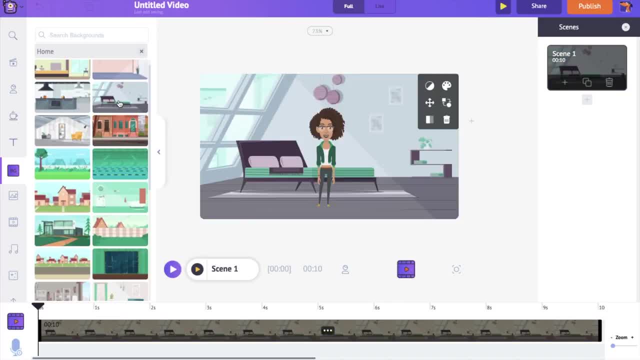 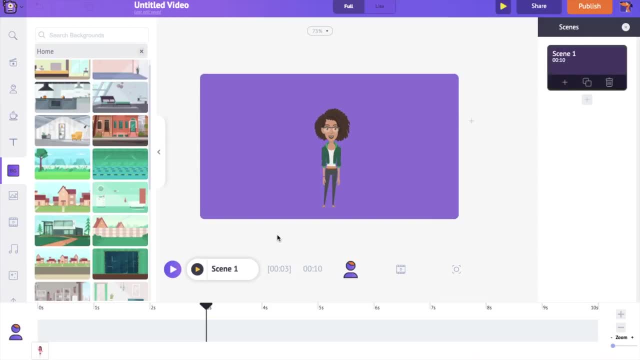 applied to the scene. I am fine with the colored background that we created earlier, so I'm deleting this 2d background that we applied. now let's see how to add text to your videos. to add text, open the text section of the library and click on one of the text. 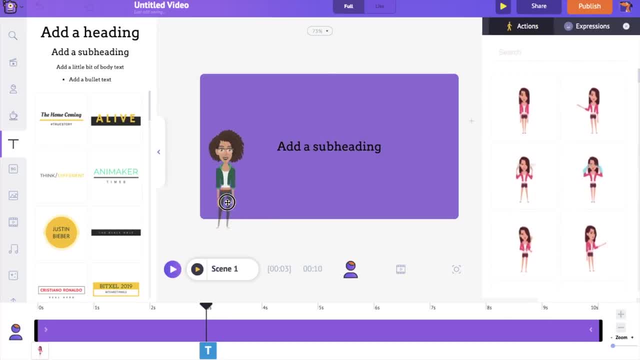 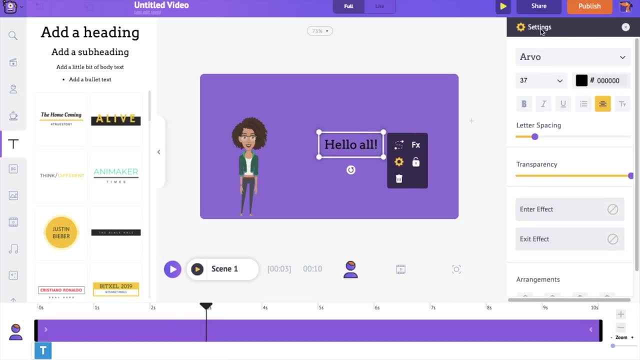 boxes at the top. now type in the text in the text box. over the workspace on the right hand side you can notice the settings tab. from here you can customize the text. you can change the font style, size, color, spacing and even transparency to apply animation effects to the text. 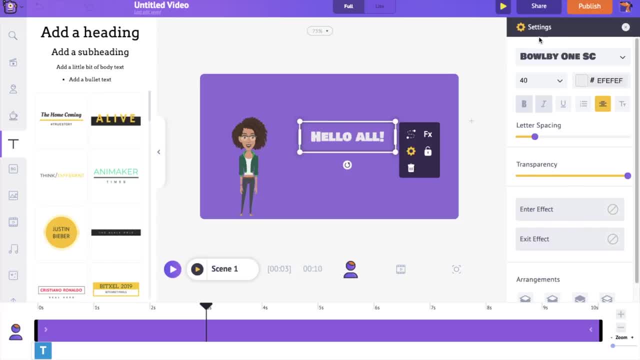 we have two options, named enter effect and exit effect, at the bottom of the settings tab. if you further click on the enter effect option, you will get a lot of different enter animation effects that can be applied to the text. once you click on an animation effect, you can notice a new pink colored part in the 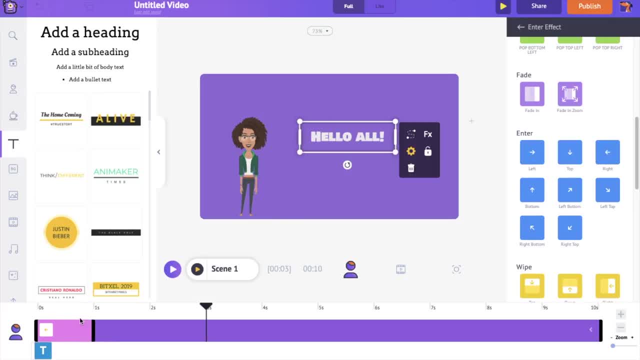 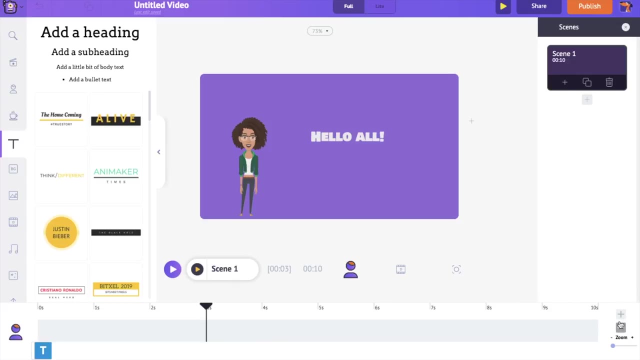 timeline. it indicates the animation effect that we applied. now you can increase or decrease the duration of the animation effect by increasing or decreasing the length of the pink part in the timeline. if you want to increase or decrease the duration of a scene, you can do that by using these plus and minus icon over here on the timeline. the plus option will. 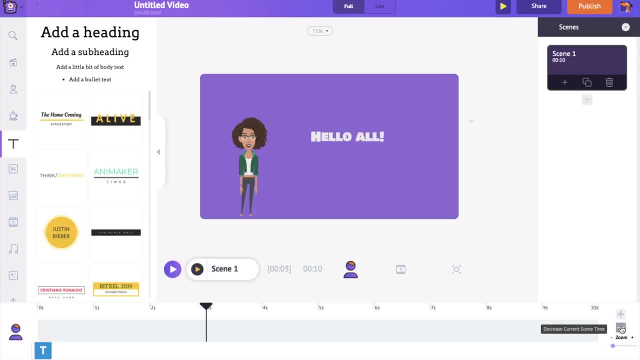 increase the duration by one second and the minus option will decrease the duration by one second. right now, the duration of the scene is 10 seconds and I want to reduce it to five seconds, so I'm using this minus icon over here to reduce the scene duration to. 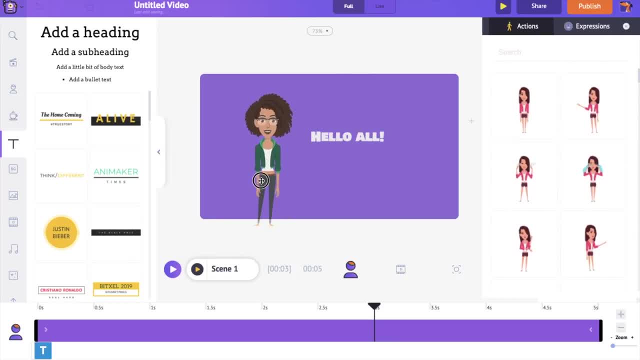 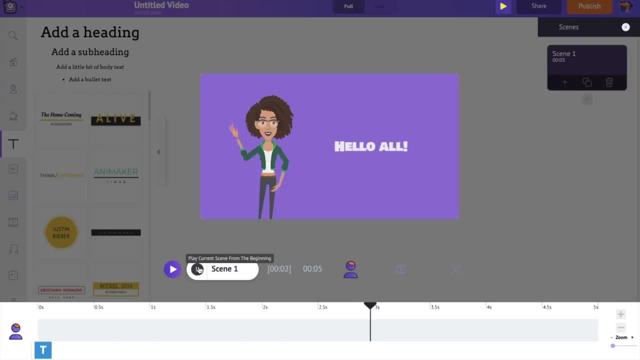 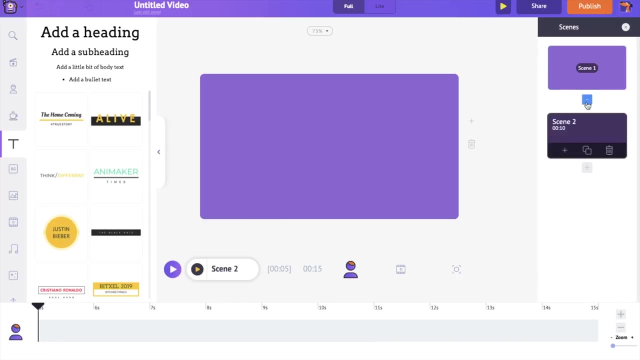 five seconds to create a new scene. go to the scene section and click on the add scene option over here. you can also duplicate the current scene and edit over it using the duplicate scene option over here and also delete a scene using the delete option. now you know how. 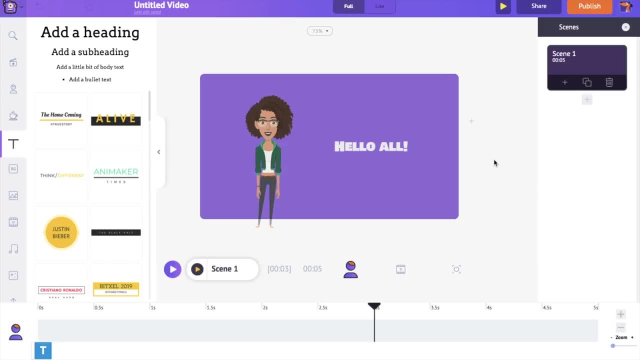 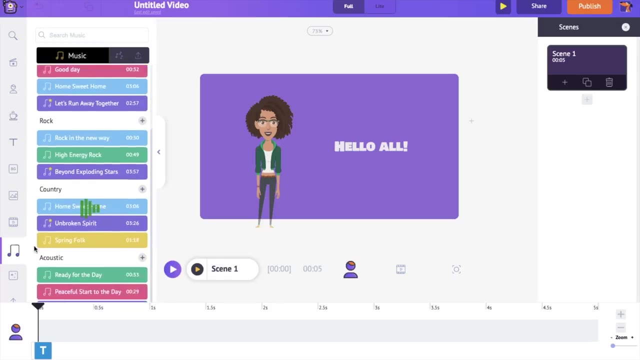 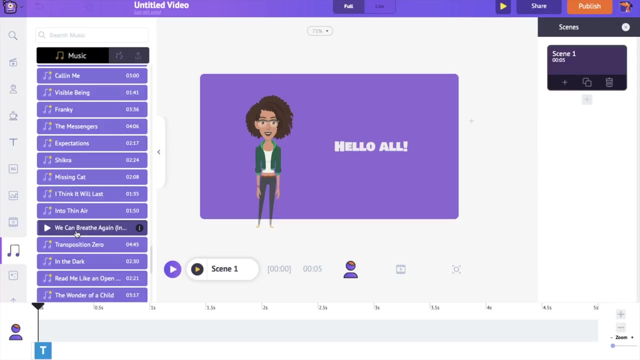 to successfully create a scene, create multiple scenes, add your custom character, add the text and complete your video. if you want to add music to the video, open the music section in the library. you can find more than 30,000 copyright-free music tracks over here. to have a preview of a track, keep the pointer over it. to use the track: click. 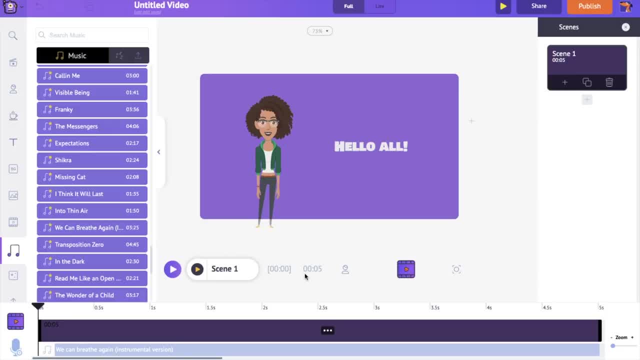 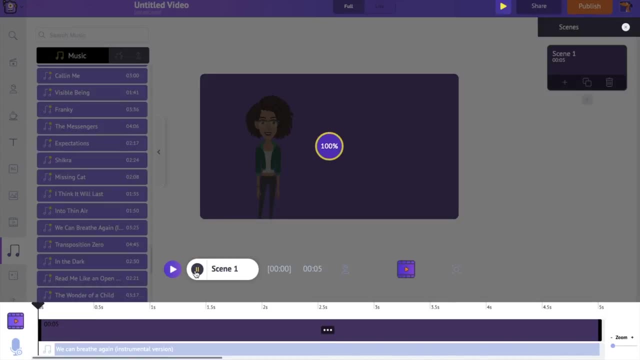 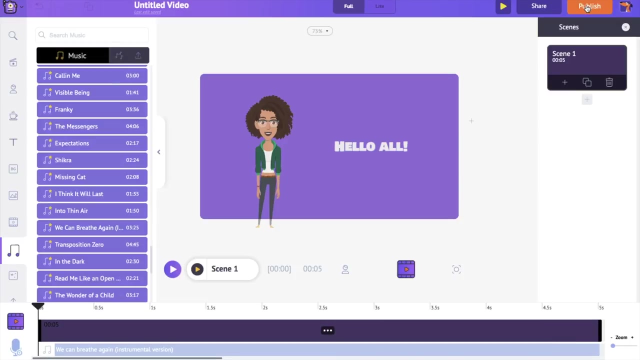 on it. now you can see the video timeline with the music track added to it. if you further select the track on the timeline, you will get more options. you can preview the track, control its volume, duplicate it and delete it. to download your video, go to the publish option at the top, click download video and